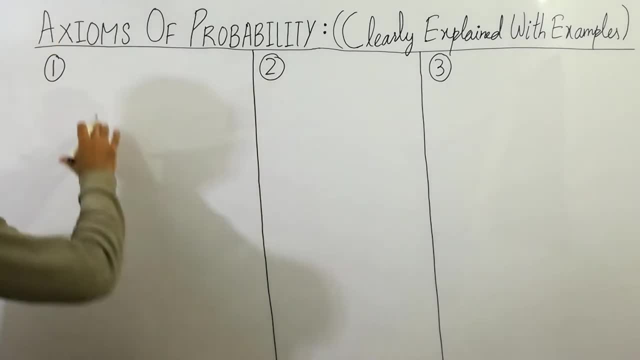 Let's start the lecture. First of all, I am going to discuss the first example of probability. This lecture is not available in any part. This will clear you all concepts. First of all, let's suppose that we have A. You can see that A is an even 1,, 2,, 3.. Let's suppose that it is the even. 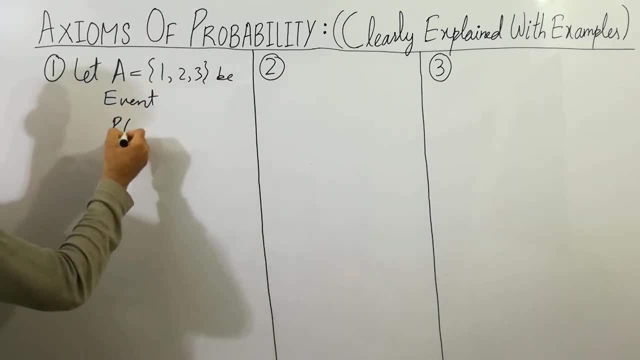 You must remember that probability of A- you can say that probability of an even is- always lies between 0 and 1.. What means that? What means that probability of A lies between 0 and 1? How, How to prove it. I will discuss the examples also. 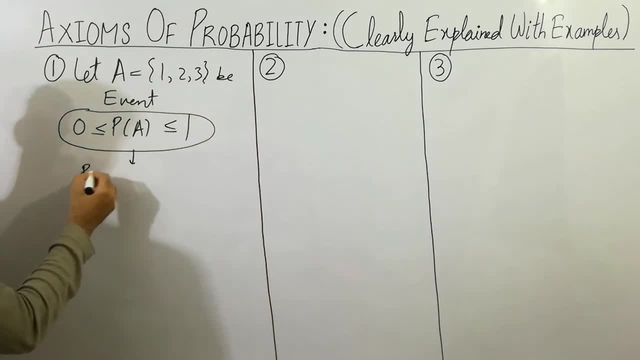 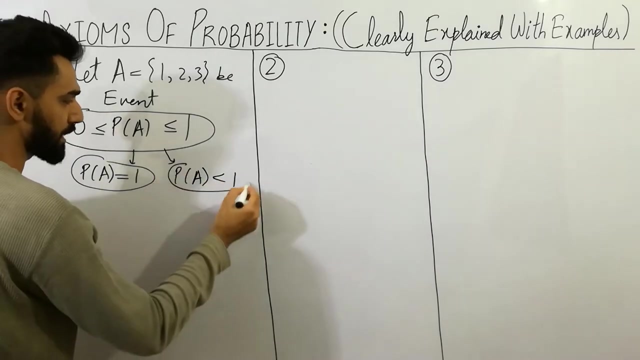 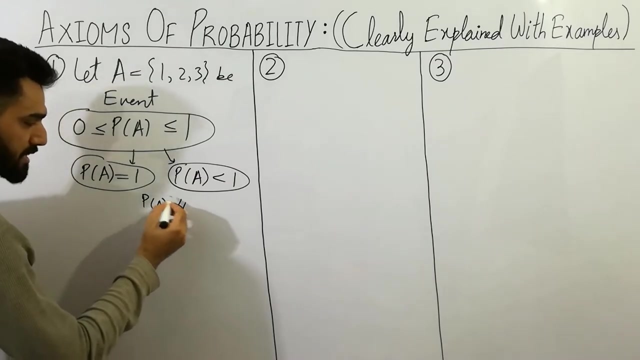 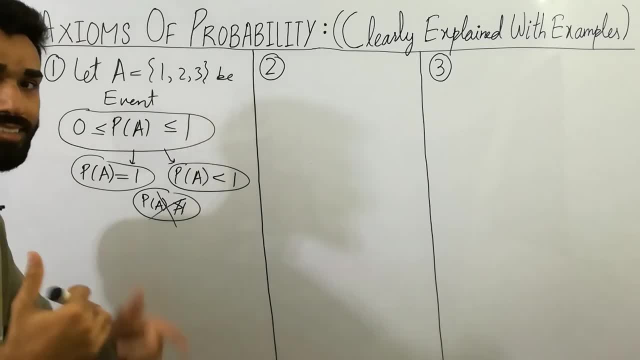 remember- this is the first point and just discuss the example. so let's discuss the example here that we cleared all concepts about probability and it made easy, so let's let's move that. probability of a s is the. you can say that for one dice. for one dice, you can say that s, which is. you can say that: 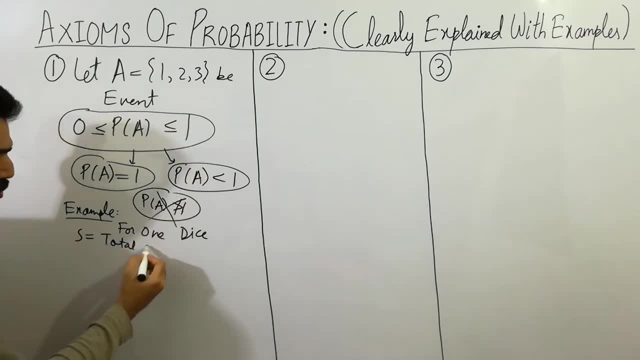 total sample space. s is our total sample space, total sample space which is here: one, two, three, four, five, six. we know that dice has a six sides. now I'm going to calculate that how per value is equal to one, how by U less than one. I'm going to prove that with example200, a. first of all, I'm going to 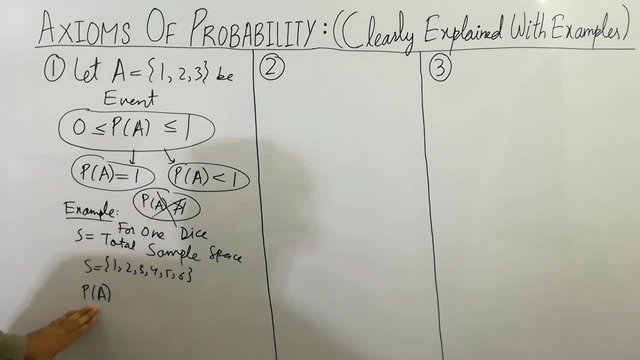 calculate the positive effect probability of A. what is the probability of A? what is the probability of an event? it's always equal to number in A. this shows that number in an event, A divided by number in total sample space. that's clear, so you can hear: A is given here one. 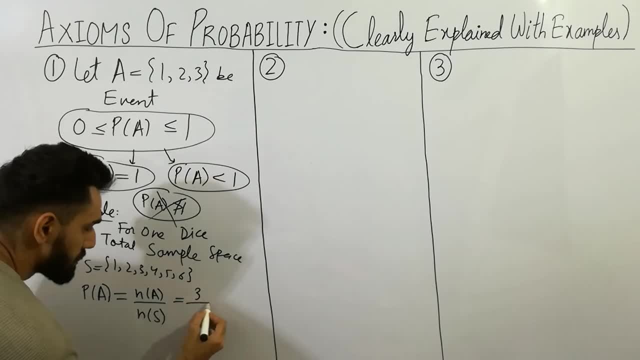 two, three. counter values are three values. number in sample space: one, two, three, four, five, six. we're going to calculate: 3 x 3 equals to six, 1 by 2, which is equal to 0.5, which is less than 1. so I prove that probability of A is. 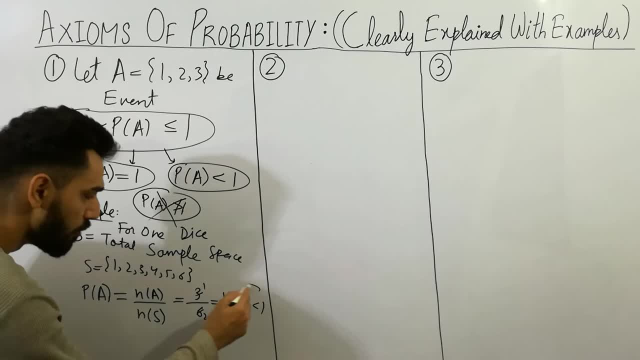 equal to 1, or you can say than less than 1, but can't be greater than. I hope that you have clear the first exam of probability. I hope that this is very, very easy. now I'm going to move to the second exam. now I'm going to move to the second exam. 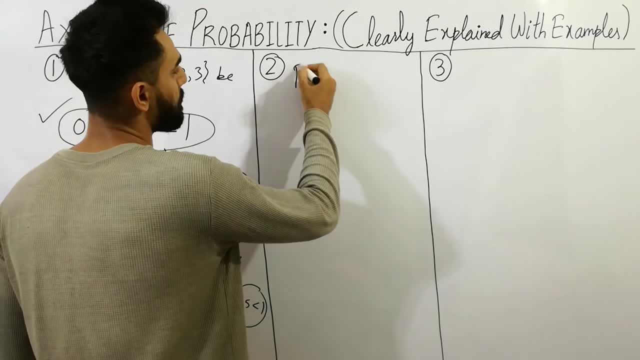 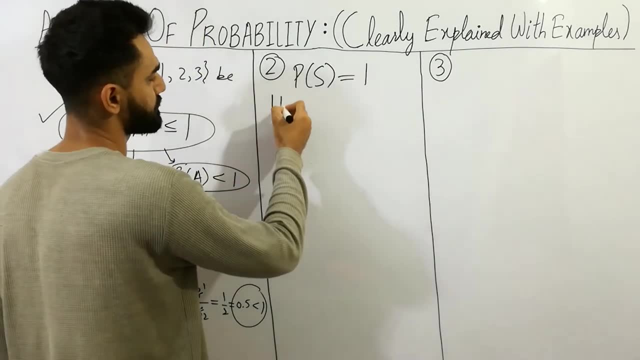 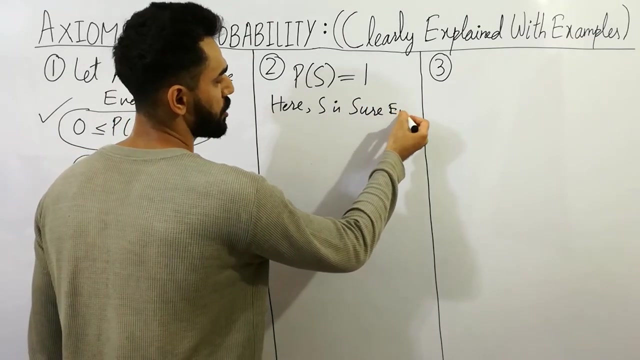 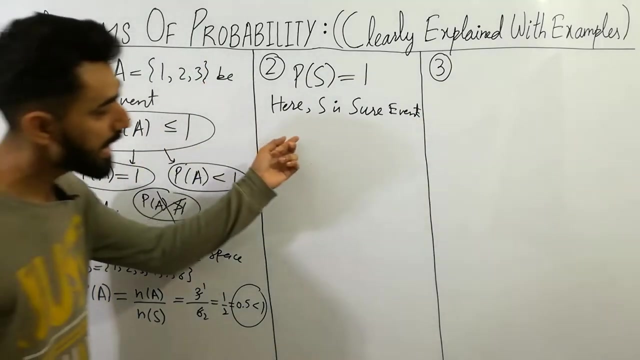 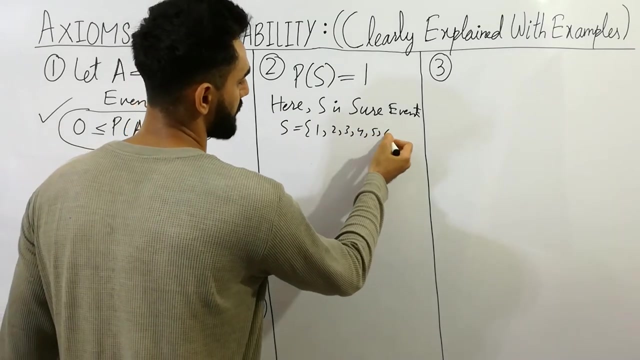 will also clear your concepts. this is probability of. s is always equal to 1. how what is s? here? s is a sure event. s is a sure event, not a sample space. this is the. s is a sample space, but here s is our sure event. you can say that s is equal to 1, 2, 3, 4, 5, 6. this is just like the sample space. 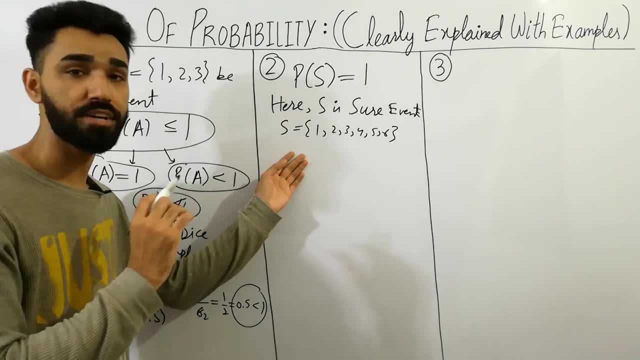 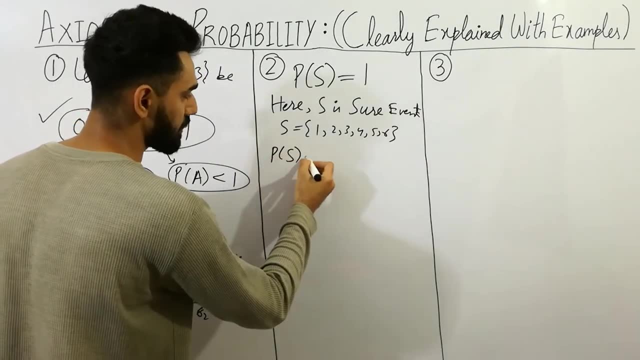 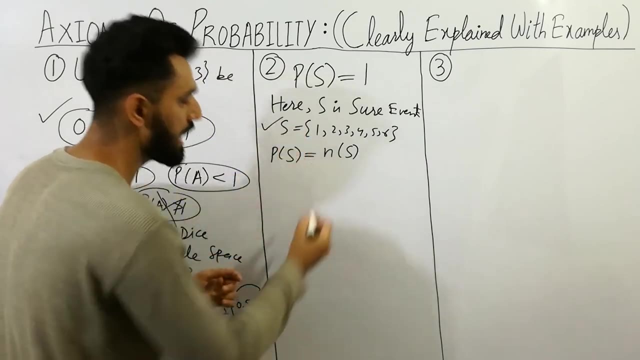 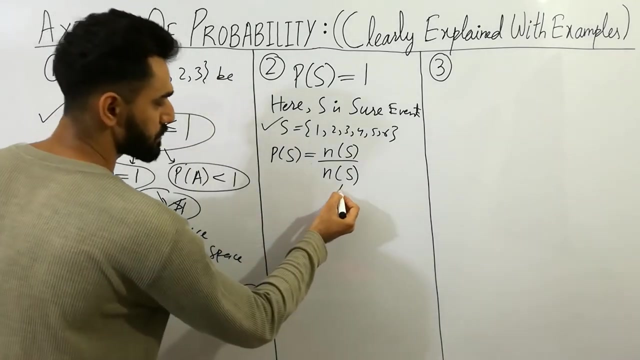 but here, in this exume, s is showing here any event, not a sample space, that's clear. so here, probability of s, you can easily calculate. probability of s is equal to number in an short event, which is s and divided by number in total sample square. this is the, this is the total Memphis and this is total sample space. 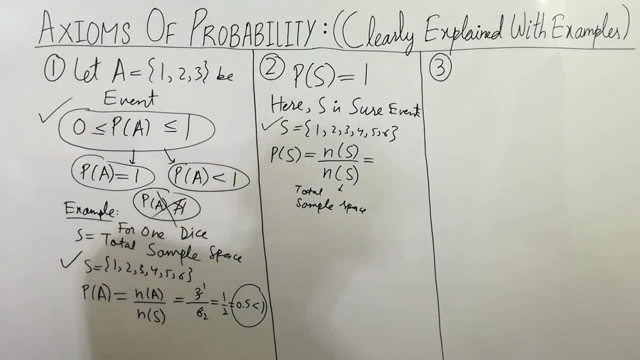 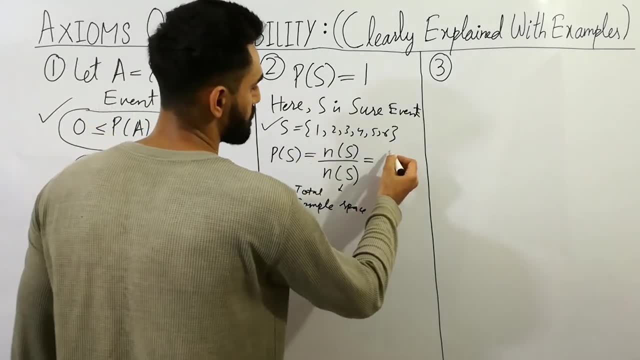 now going to calculate. here number is sample space, so here number is sample space. are chain 1, 2,, 3,4,, 5, 6, so here I put a s over here and it's total sample space. what is the total sample space? total sample space is here: 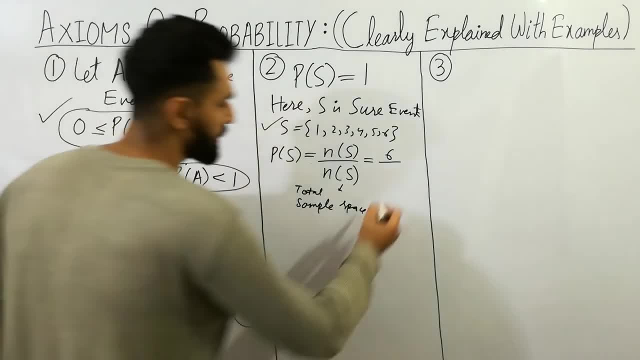 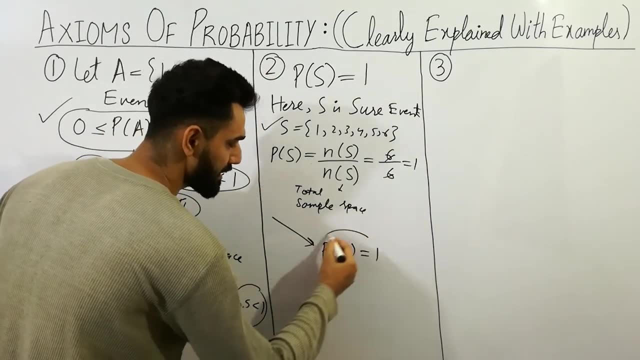 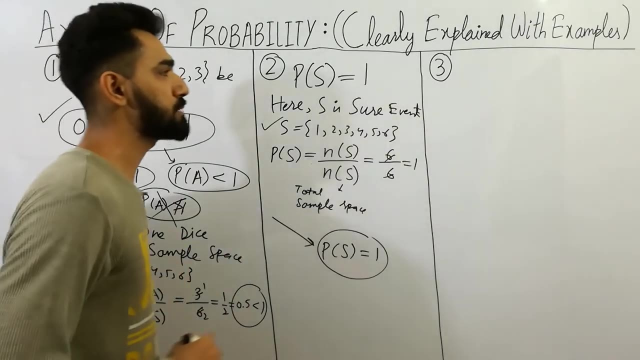 1, 2, 3, 4, 5, 6 for the six best. yes, it will be easy. so here I prove that probability of s is always equal to 1. this is the proof. I hope that we have cleared the also second example of probability. next I'm going to move the last example of probability. 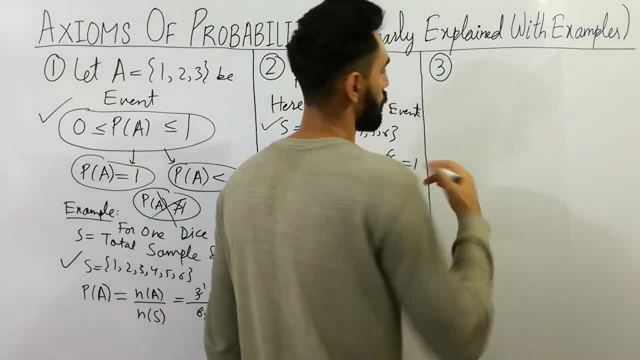 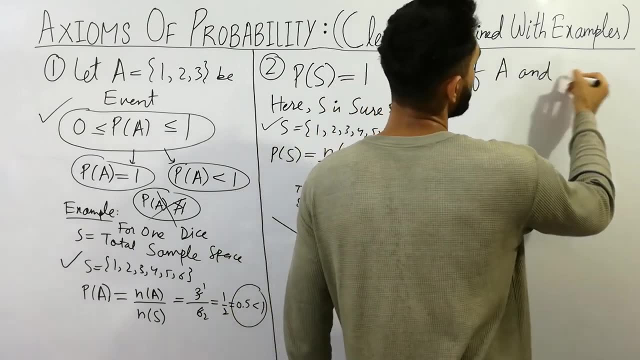 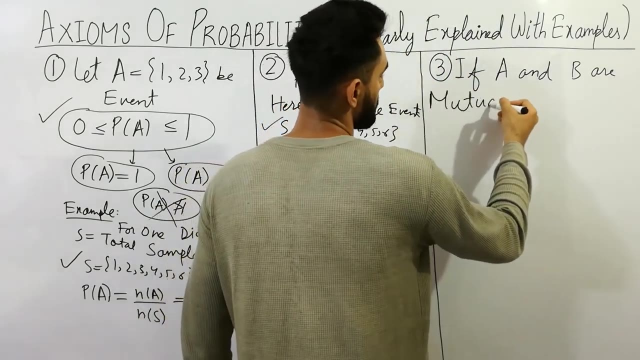 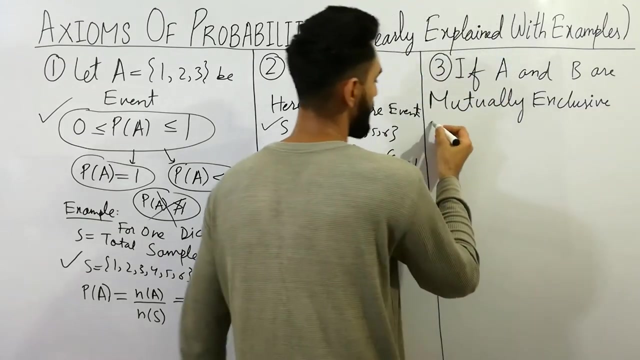 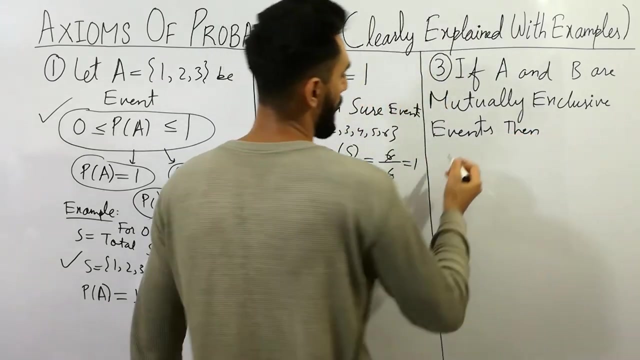 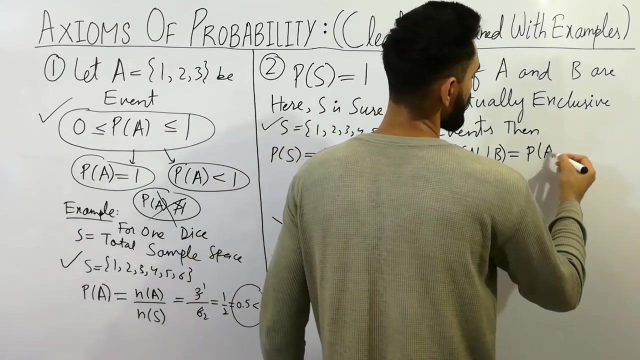 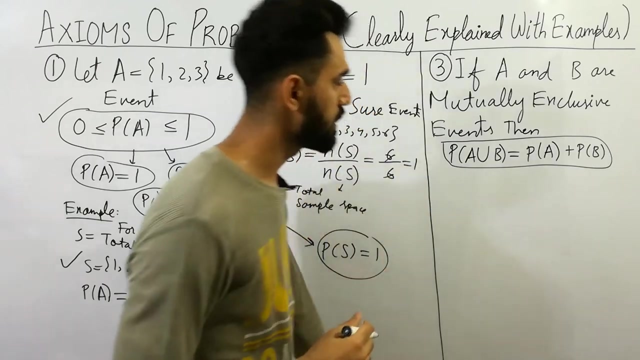 this is also clear in all concepts. so here, third, what is the third example? if A and B is A and B are mutually mutually exclusive- viewers, mutually exclusive ever- then must remember that probability of a union B is always equal to probability of a plus for bank of B must happen now. first step is here: what are the mutually exclusive? this is: 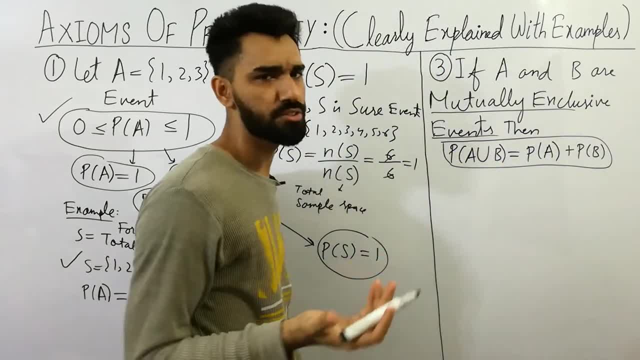 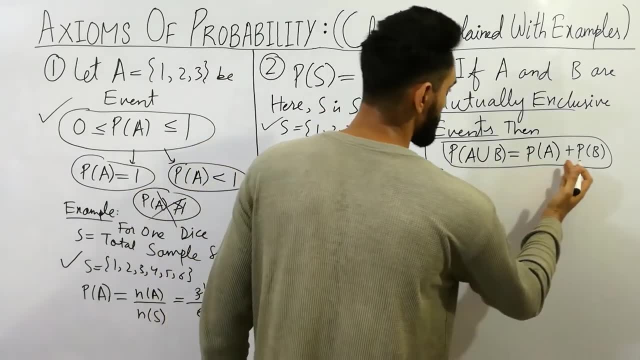 a main point: what are the mutually exclusive words? let's take that example and also I'm going to prove that value of A and B is equal to value of A plus value of B. I'm going to prove also with example. now the lesson is the example. so 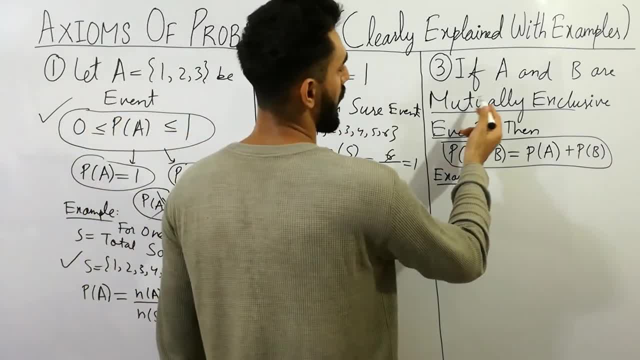 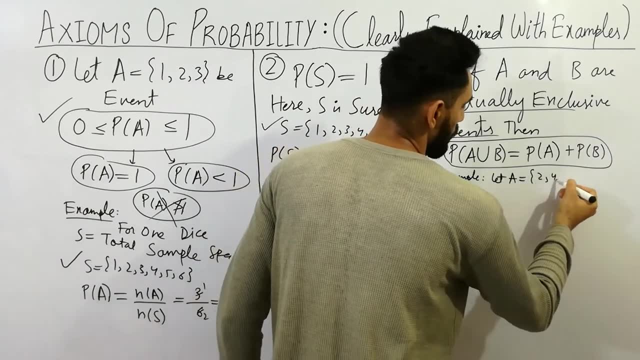 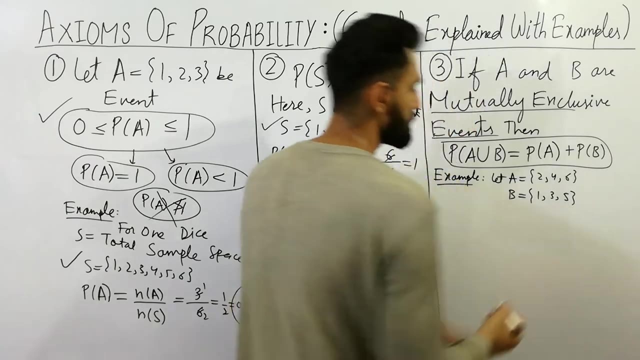 here but are. the first point is here how A and B, but is mutually exclusive. let's suppose that A is equal to 2, 4, 6 and you can say that B is equal to 1, 3, 5. this is the even number, this is the odd number, but means that mutually exclusive means. 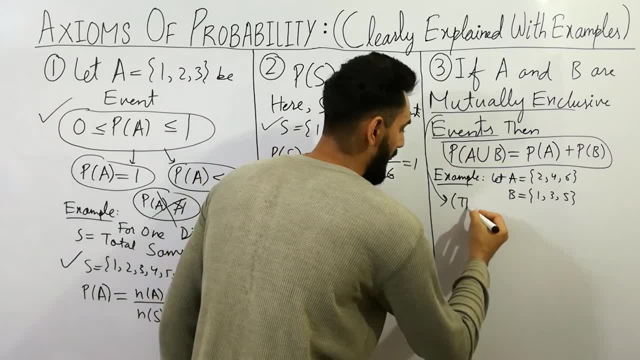 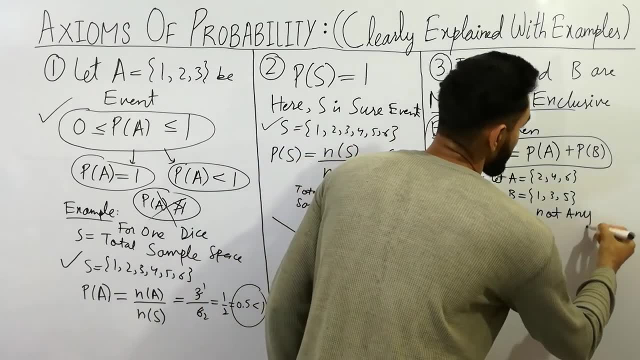 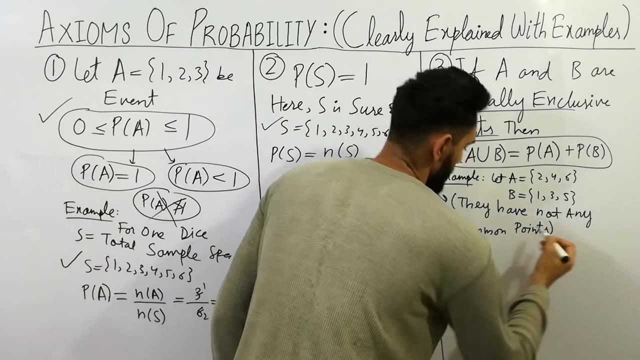 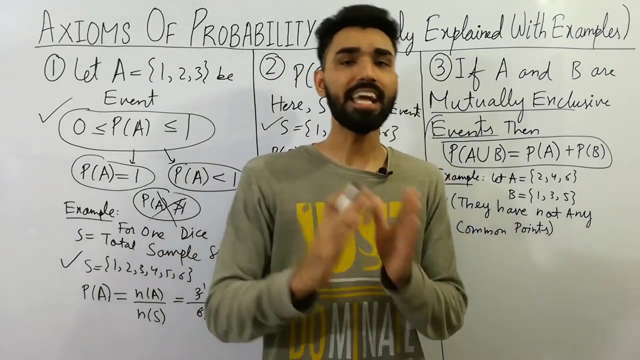 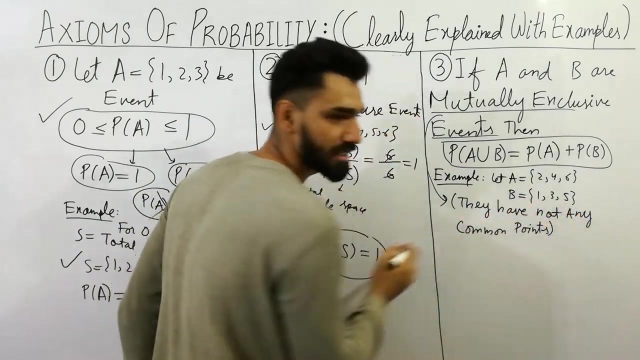 it means they have not any common points and must remember that. but what are the mutually exclusive? ever you can say that if A and B are no common points, that content, which resource does this consider? head is true. here is true, is naughty. one head is for a poor, is not you. Elexus says: here is one, but here one. 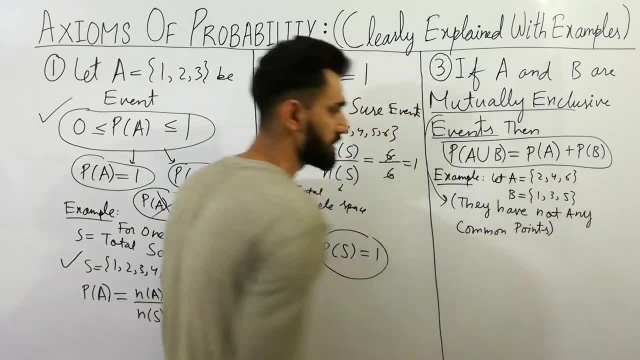 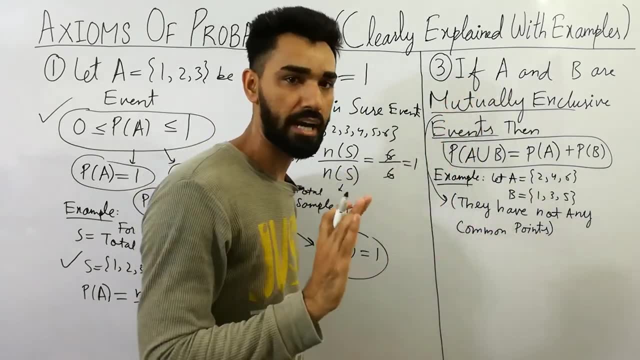 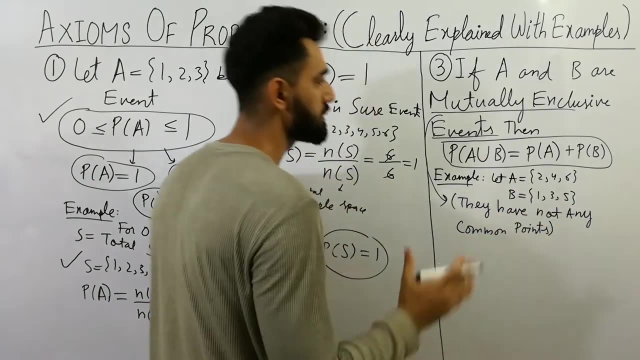 is not- cables. here is three here. three is not given. that's for that. they have not any common points. that's called as mutually exclusive. I hope that you are clear at the point. but are the mutually exclusive? even? they have no common points. they are not matching together. that's called as mutually exclusive. even now I'm going to. 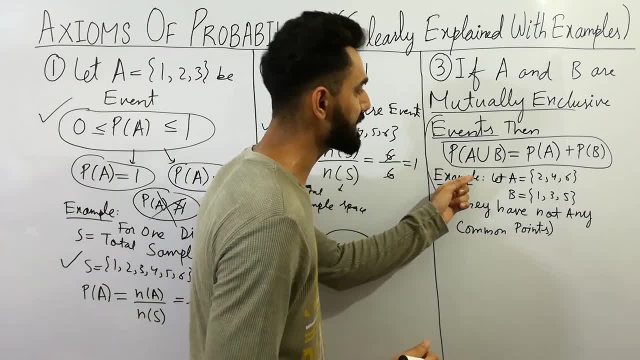 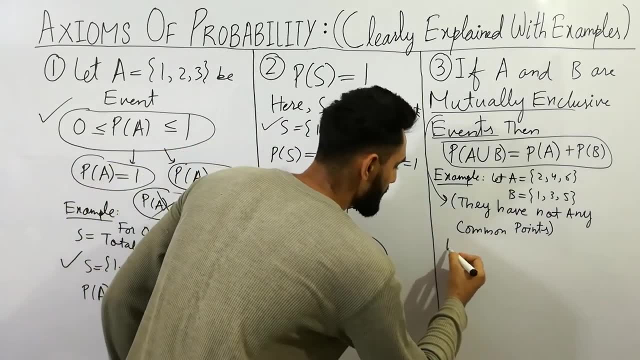 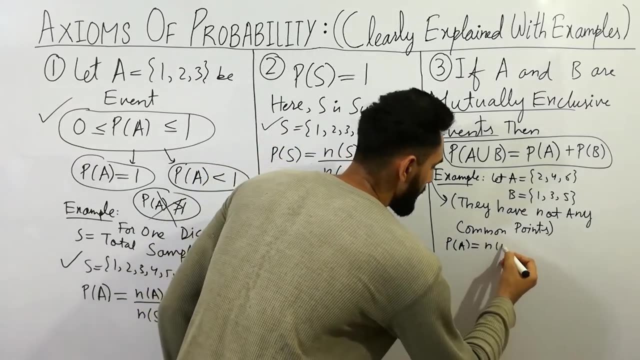 prove that, how probability of A union B is equal to probability of A plus probability of B. so I'm going to prove that. so for next student, probability of a, let's going to calculate Class. probability of a is equal to number in A divided by number in sulfur space. so 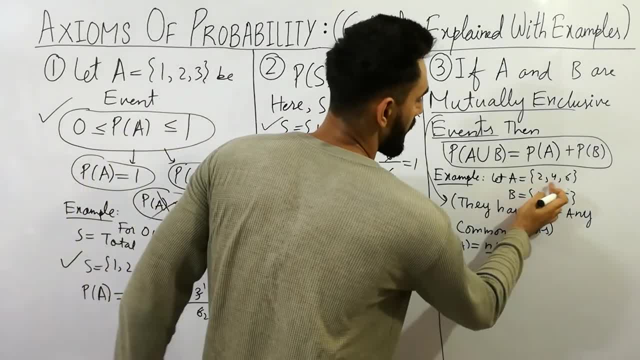 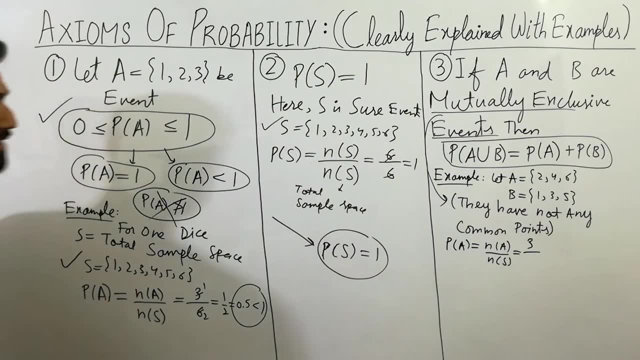 here number in A is given as 1, 2 or 3. 3 divided by total sulfur space and a total sample space is 6. so here I put: 3 is equal to 0.5. here 3 is equal to 0.5. 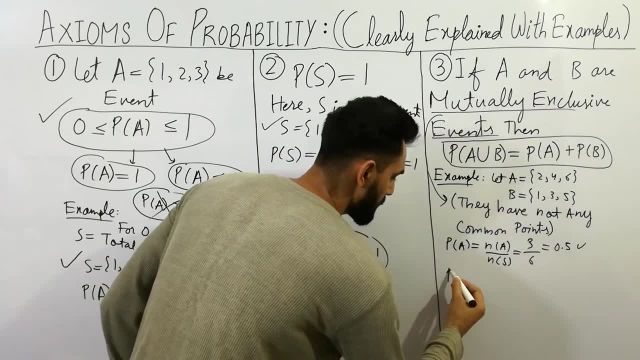 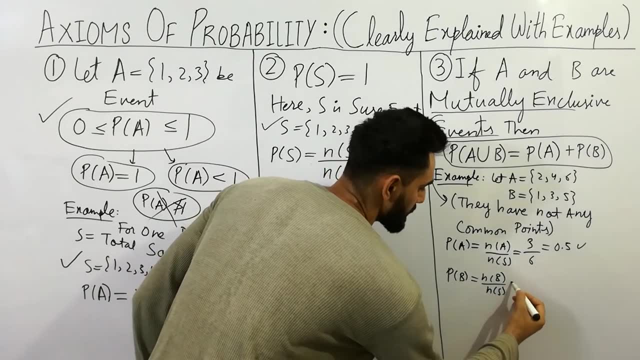 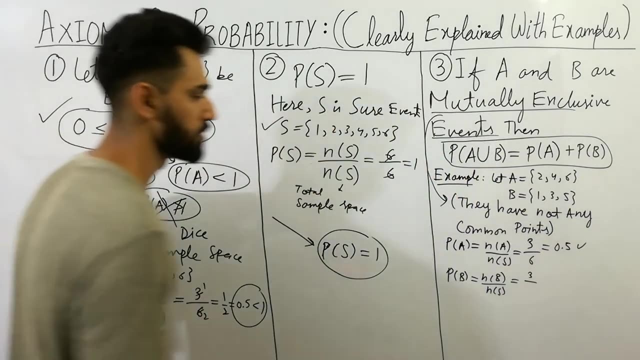 That's clear. Next point: Now I'm going to calculate. probability of B is equal to number in B divided by number in sample space. Here B is also 3. numbers 3 over total sample space is also 6.. Supporting end will get also 0.5.. That's clear. 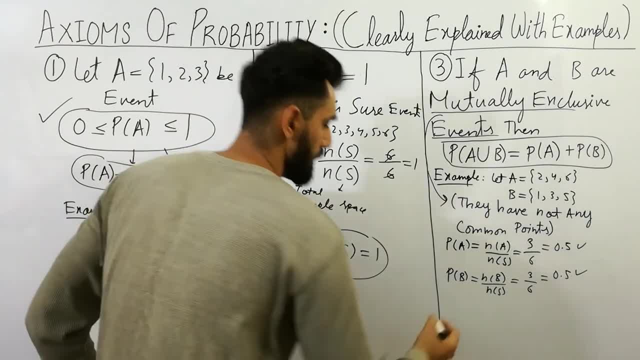 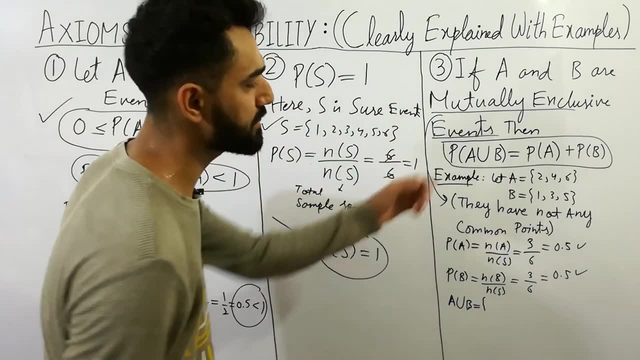 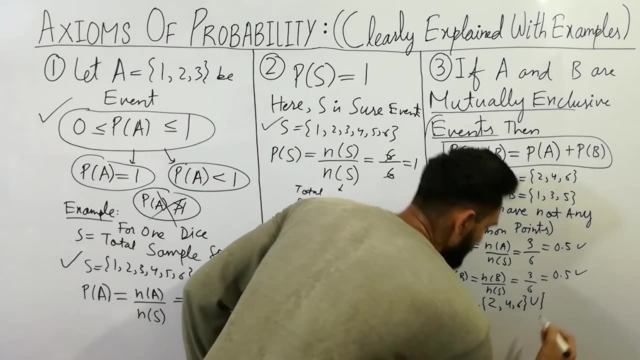 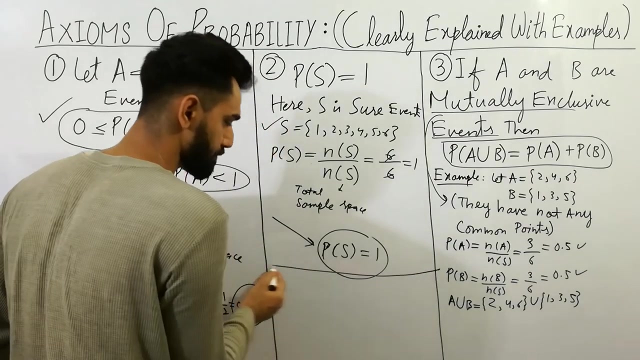 Now next step. Now next step is here: A union B. Now I'm going to calculate here: A union B. So here. A is even here. A is even here: 2, 4, 6.. That's clear Union. Next step is here: B: 1, 3, 5.. So here. next step is here, simply. Now I'm going to calculate the union here. 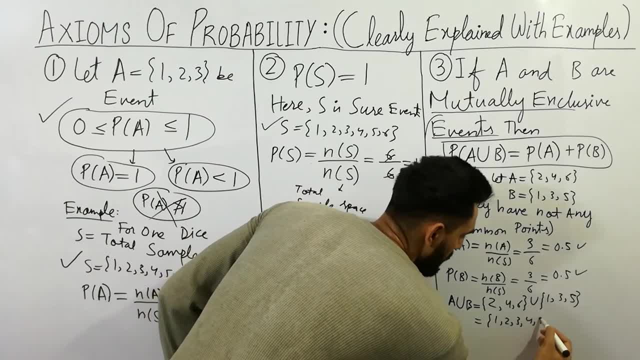 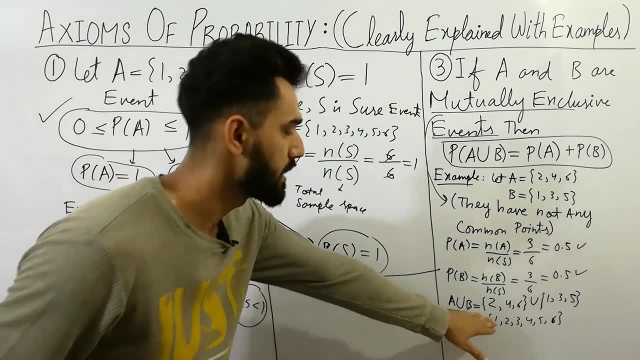 1,, 2,, 3, 5.. 1,, 2,, 3,, 4,, 5,, 6.. So here A union B is equal to 1,, 2,, 3,, 4,, 5, 6.. Now I'm going to calculate that. Now I'm going to the next step.